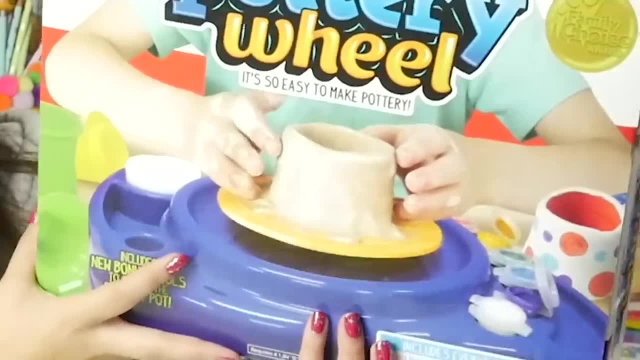 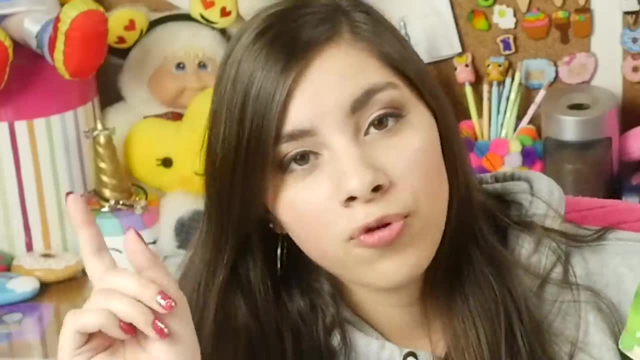 The hands on the picture look to be an 8-year-old's hands, So that gives me some hope because I'm thinking maybe I as a 23-year-old can manage it. But I'm still doubtful. We're gonna keep an open mind and we're gonna try our best. 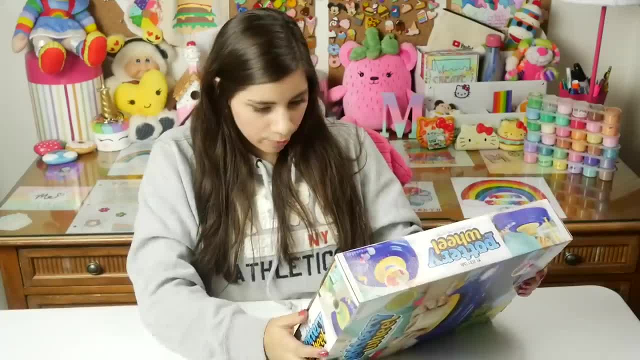 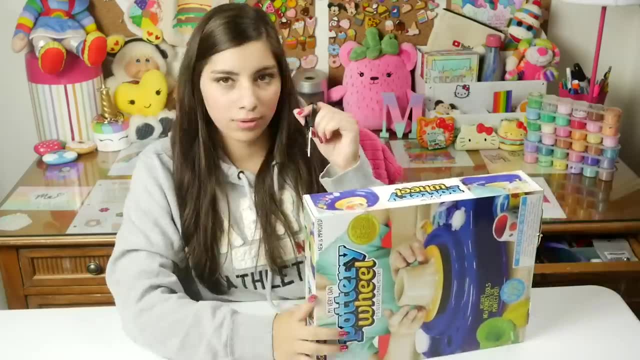 And daggone it. I'm gonna make something cute. Let's just jump into this. FYI, I'm dressed like this because I figured this would be getting messy. That's the only reason I'm gonna open this up. Let's open up this box. 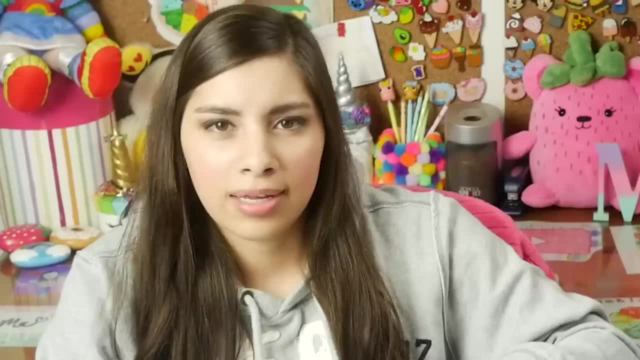 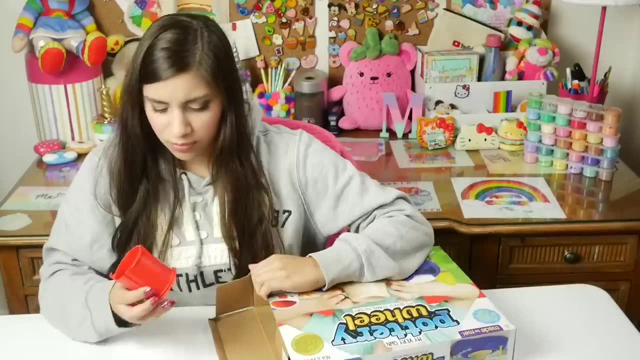 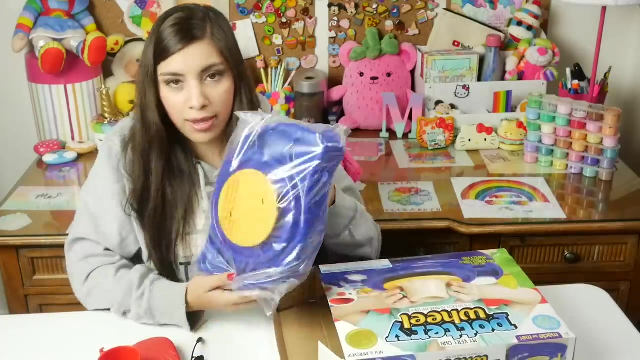 And oh, look at that, It's a box. Oh my gosh, I'm already confused. So we've got some traffic cones- Looks like some sort of button- And then we've got the big thing. This is the big thing that's gonna make the magic happen. 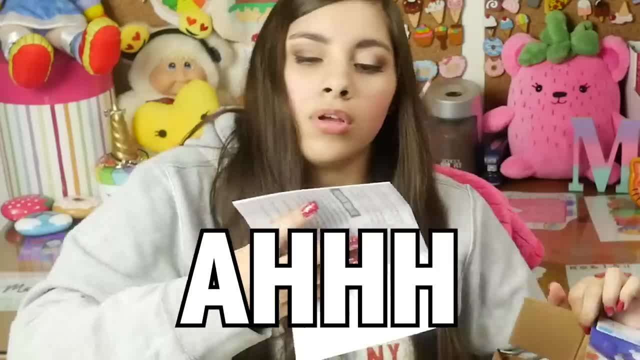 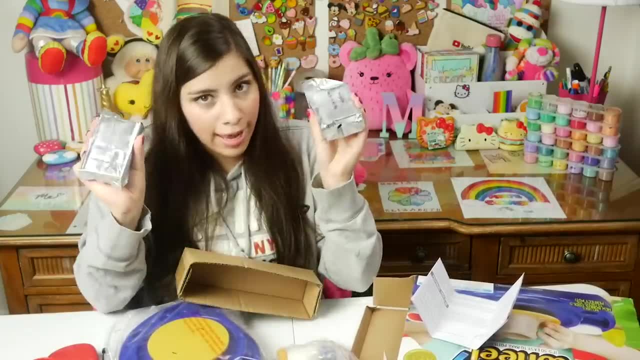 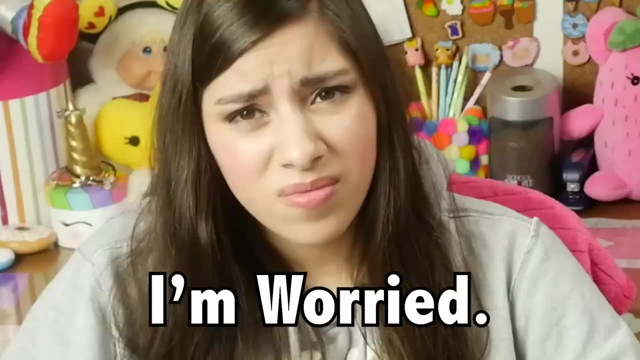 The pottery wheel. right, Right, Oh, save me please. Instructions: Packages of cream cheese. No, Um, this is the clay. Wow, that's the paint. Wow, wow, wow, wow. This is a lot of instructions. 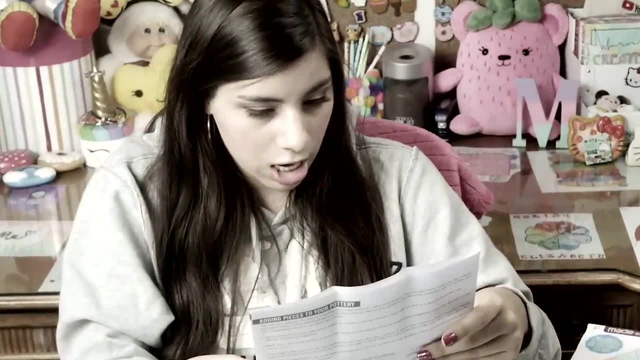 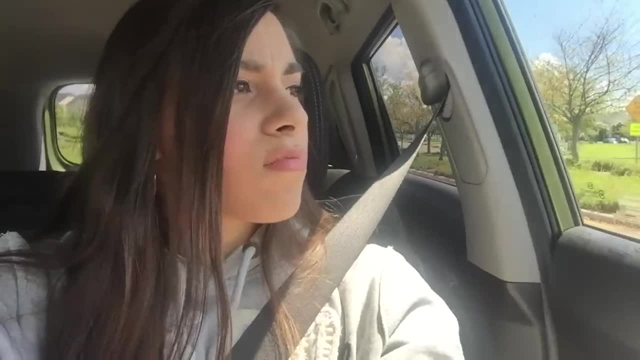 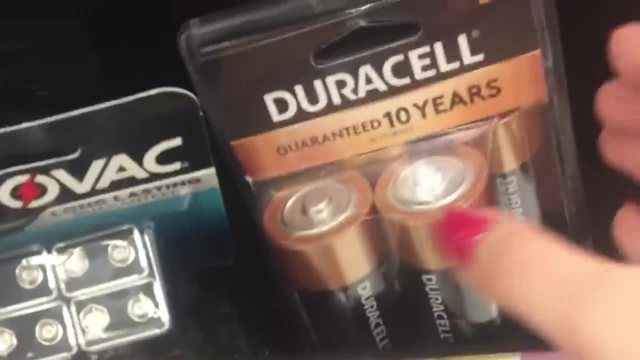 Batteries are sold separately, So I have to go. I have to go get D batteries, So I'll be back. This is new. Welcome to my car. It's so hot out here I'm gonna be all types of sweaty when I get back. 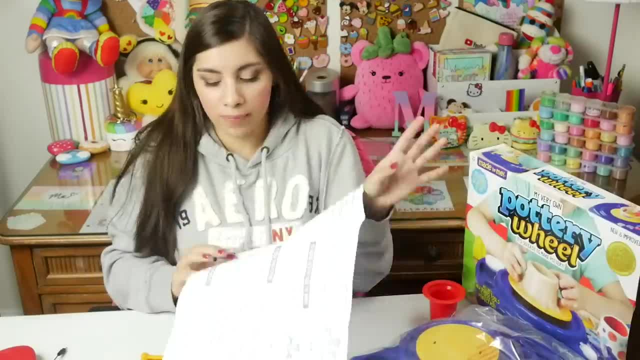 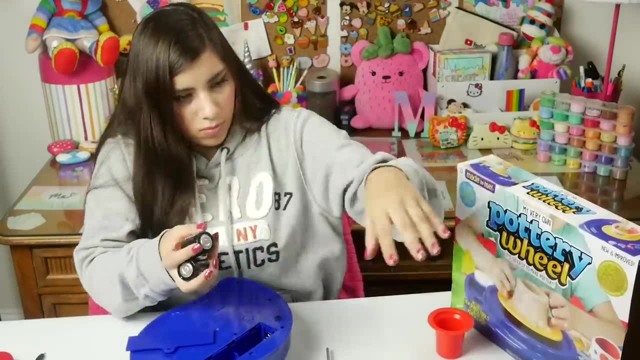 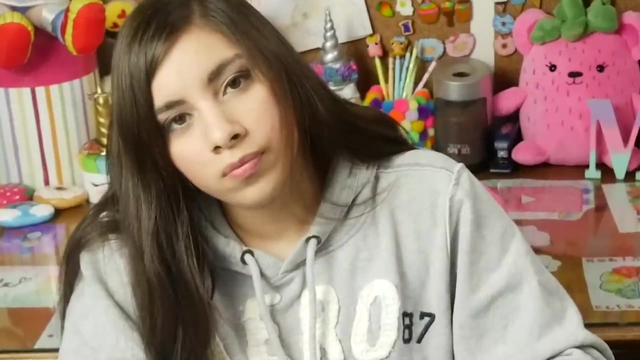 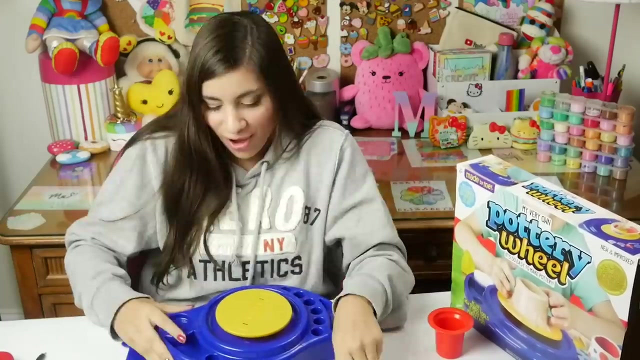 Okay, I'm back, Got the batteries. You know what I think? I kind of get it. Let's just, let's just try it and see First batteries. Okay, Okay, okay, Let me get organized here. 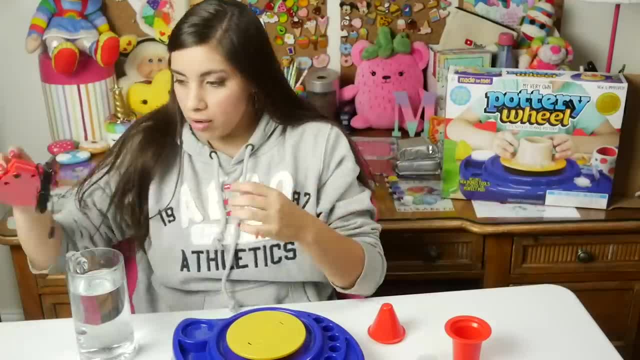 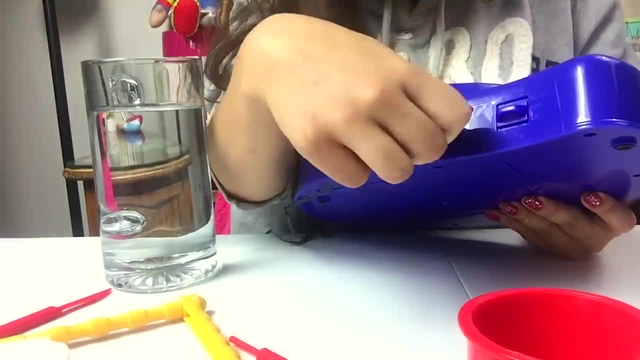 Do I want to use the pedal? I think I want to use the pedal. There's a little place where you plug in the pedal. Clay Open Half of one of these bars First before you do anything. 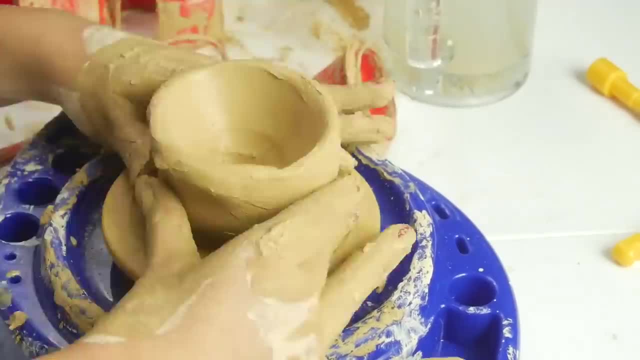 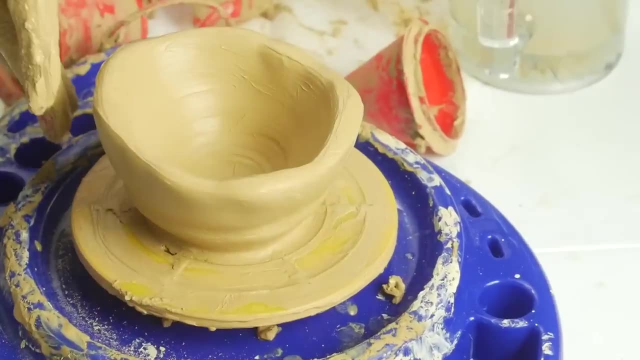 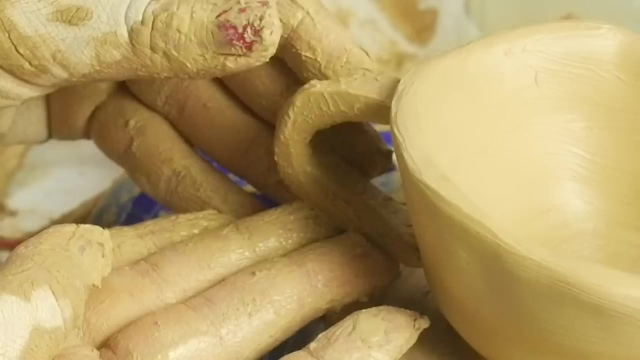 make any progress. the plate is also really, really wobbly and i just don't have the skill to overcome it and make it work. so this is what i got: train wreck. it's supposed to be a teacup, so i made a little handle for it and then use the string they provided. oh and yeah, i did ditch my nail polish. 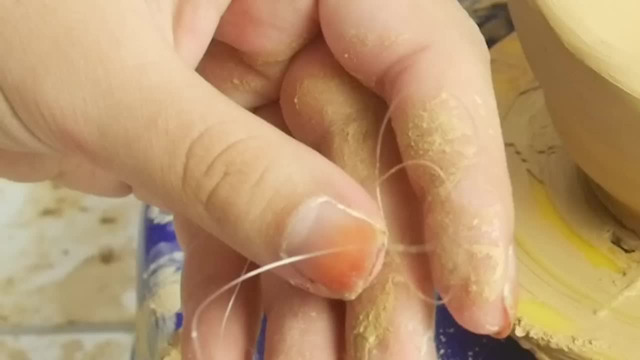 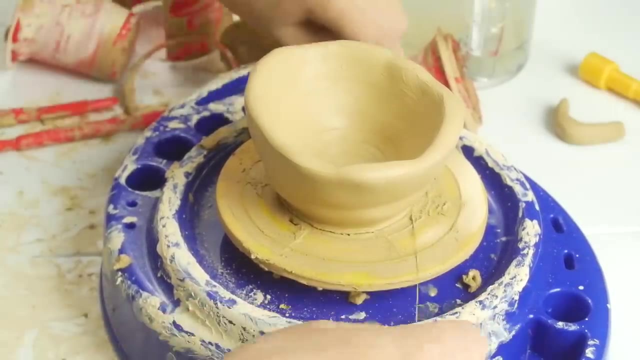 revealing my terribly stained nails, but let's pretend that that's not frightening. use the string to separate it from the plate, which did work pretty well. you probably don't have to do it that many times. okay, just stop now and then gently lift it off. wouldn't want to break that nail. 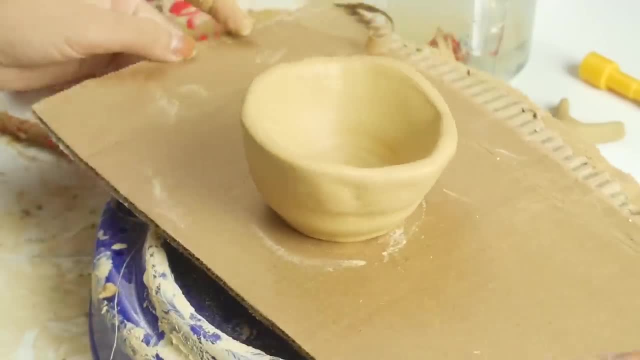 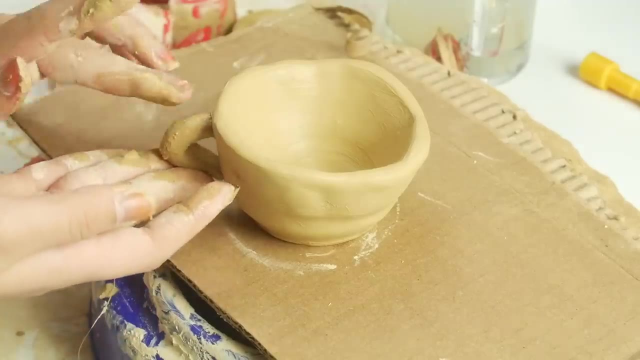 masterpiece, and now we can add the handle, and the instructions were actually helpful for this, because they reminded me to score the clay. the clay doesn't go in the oven or anything, so you're supposed to let it air dry for like 24 hours. and since i created something so lovely the first time, 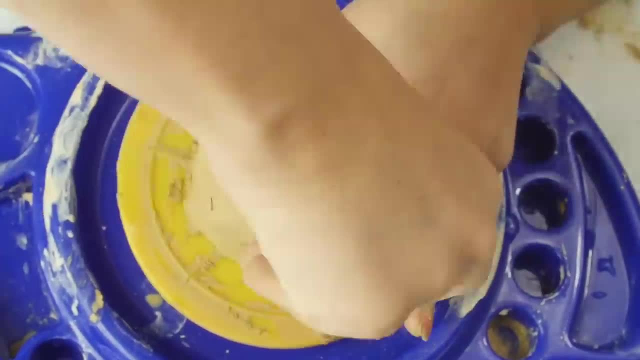 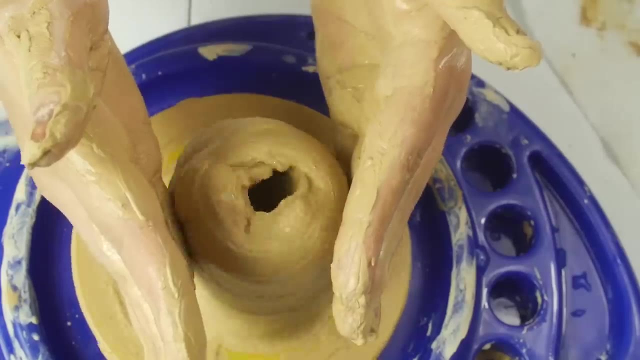 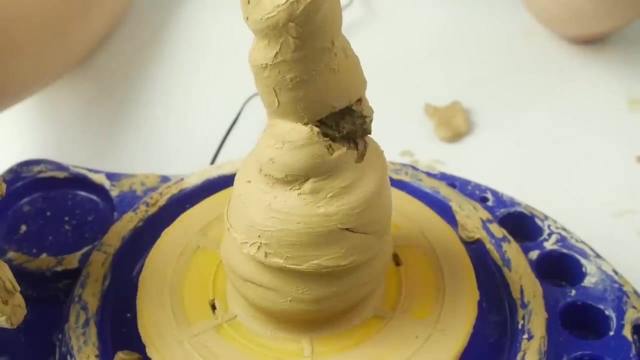 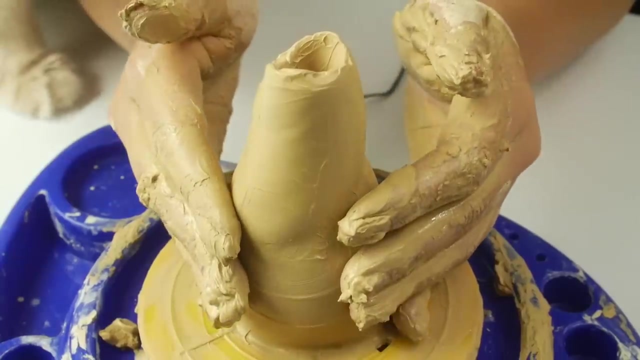 i'm gonna do it again. i was trying to make something decent literally all day, so just imagine this. for 10 hours i have had better days and i've failed at this over and over and over. what. what was i even trying to do here? i don't know. even my cat was starting to judge, but it ended up getting worse because 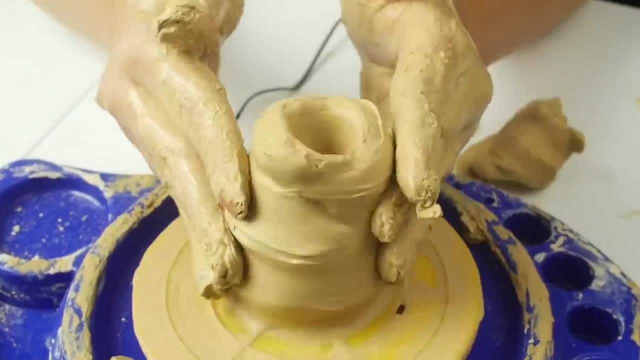 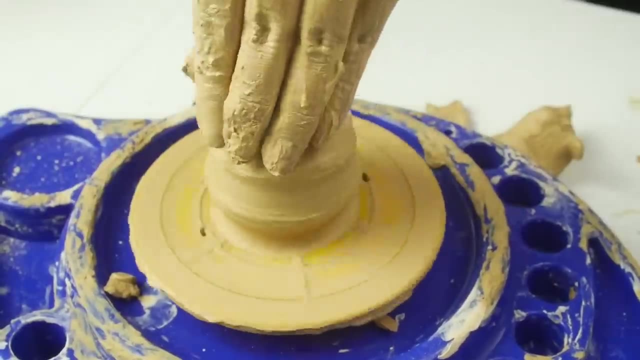 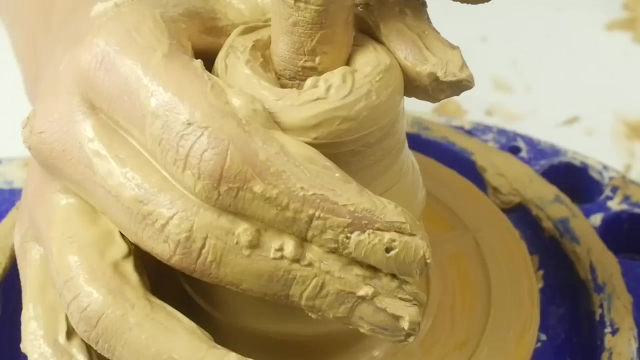 the battery started dying and it started sounding a lot like you know what i'm talking about- like it wasn't a smooth motion, so it was just getting harder and harder to get it to work. i didn't even shape. all y'all with the dirty minds cool it. okay, this is innocent. so i ended up. 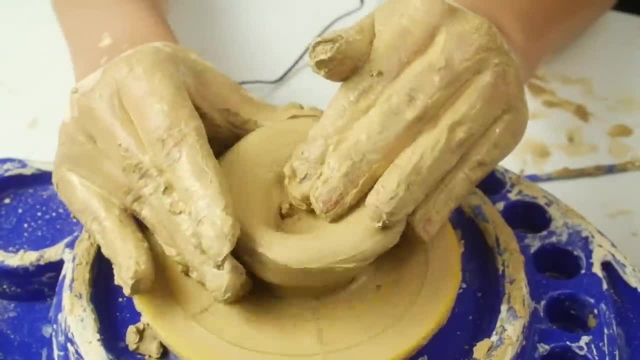 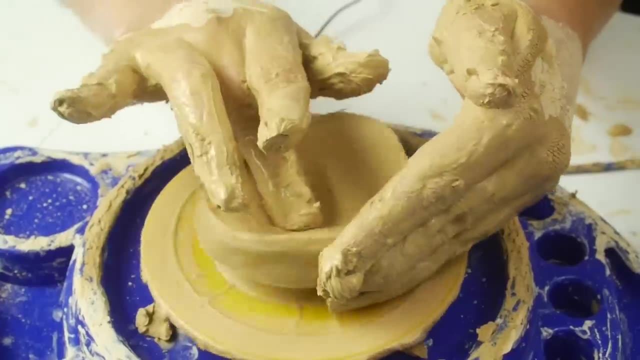 making this, and i did another one because i did want to use all of the clay that they provided. you're supposed to be able to make four pieces, but it only went far enough to make three for me, although there was probably enough on my hands for a fourth one. at this point, the battery was. 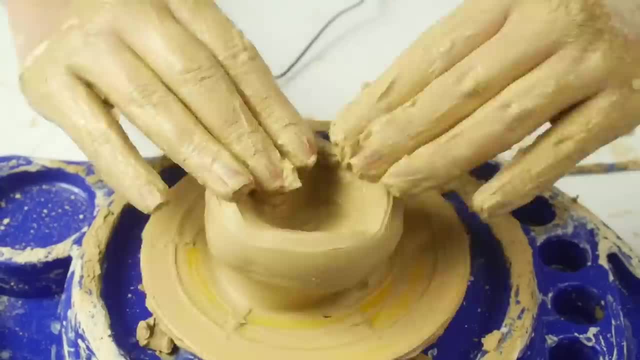 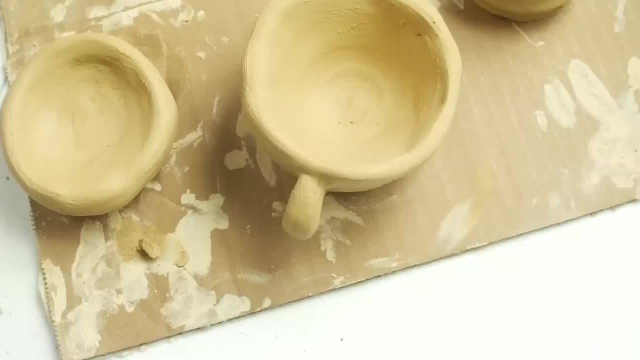 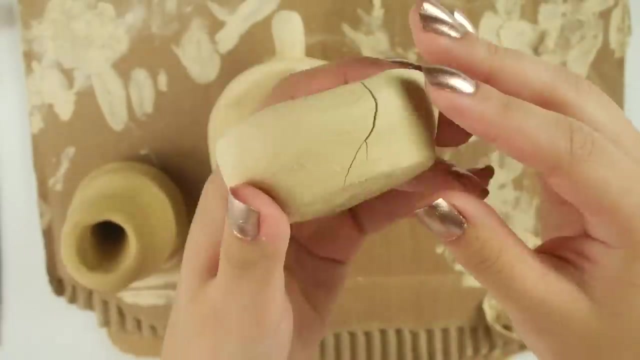 really starting to die and my spirit was dying at the same time. so this bowl is just, it's just terrible. so here are my three absolutely stunning creations that now need to dry. flash forward. it's been 24 hours and, surprise, the clay has some big cracks in it. it just gets better and better the surface. 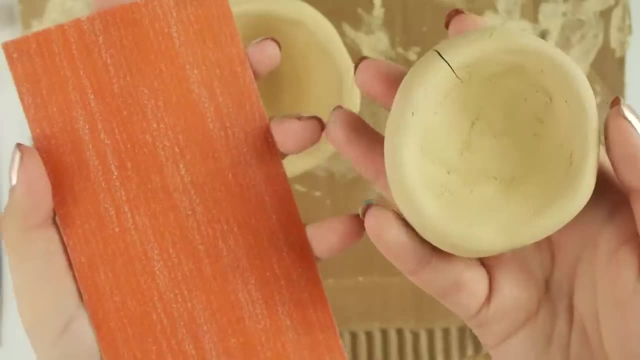 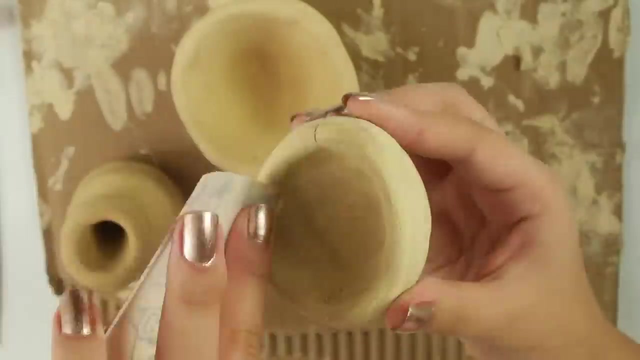 of the clay was super rough. it's got all these handprints in it, so i did use some sandpaper to smooth it out. i don't know if this is considered cheating or if people ever actually do this with pottery. i have no clue- but i was just trying to improve this in any way i could it always. 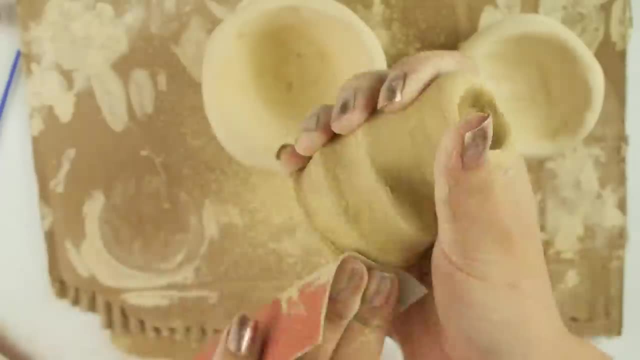 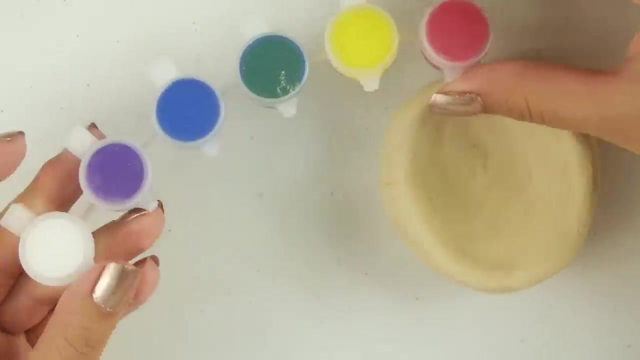 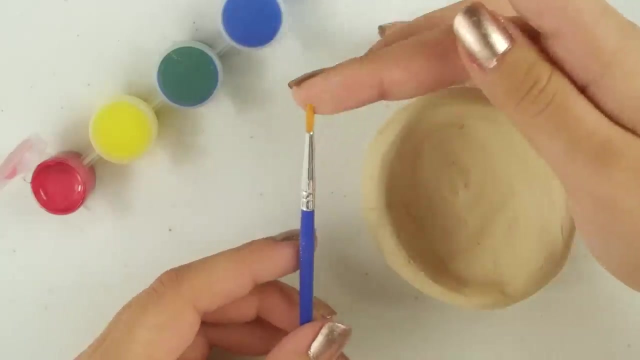 didn't help with the uneven shape, but it did help to smooth out the surface a little bit and helped with the cracks a little. finally, it's time to paint. they give you like a thimble full of each color. it's a super small amount of paint and also this really tiny paintbrush, which is fine for. 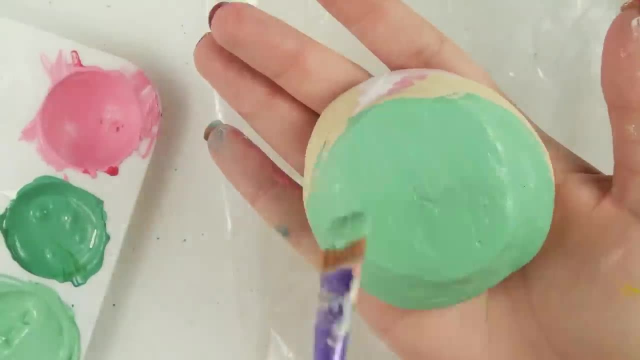 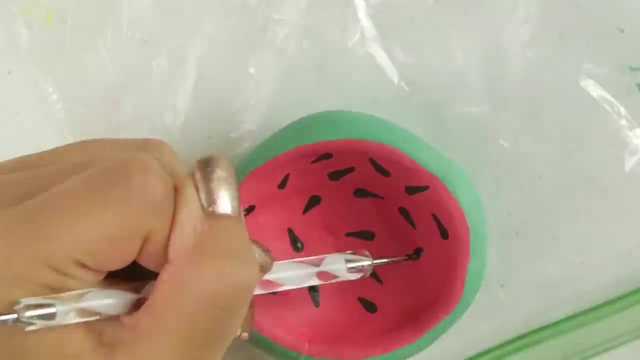 details, but it's a little annoying to use to paint larger areas. with this, i did end up using my own paintbrush and of course, i had to mix in a lot of my own paintbrushes, so i did end up using my own paintbrush and of course, i had to mix in a lot of my own paintbrushes, so i did end up using my own. 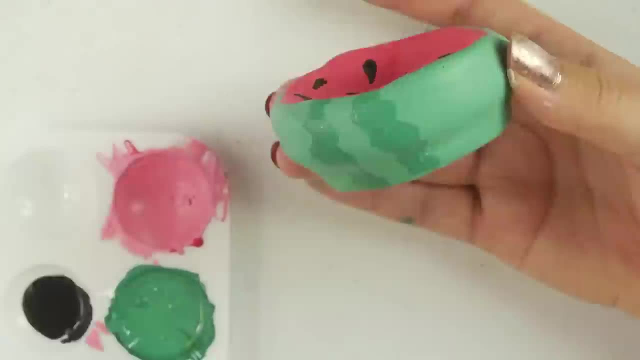 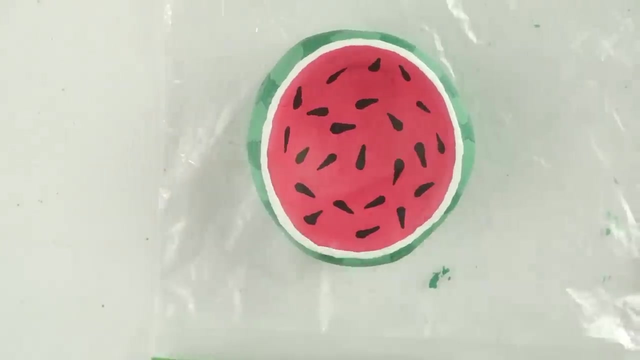 paint to be able to finish painting these. i really tried to do well on the paint jobs to make them a little cuter, but it's kind of like putting a dress on a turd. there's just not much you can really do to improve them since the shape is so bad. but you know what? let's try to be. 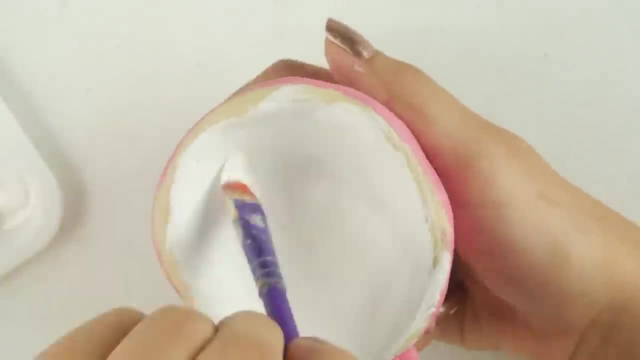 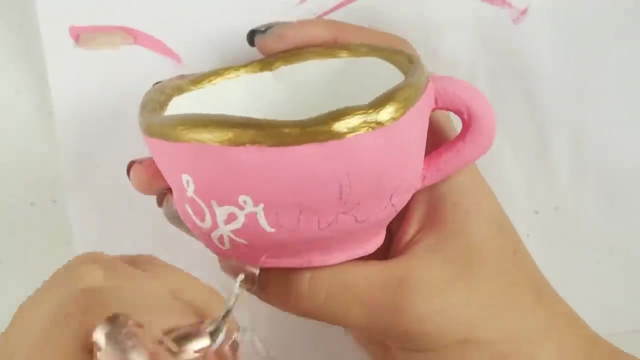 positive for just a second here. painting them was definitely my favorite part. i love painting things in general- anything really- so i did get some enjoyment from it. by the time i had painted all three pieces, i'd used every little bit of paint i had used every little bit of paint i had used. 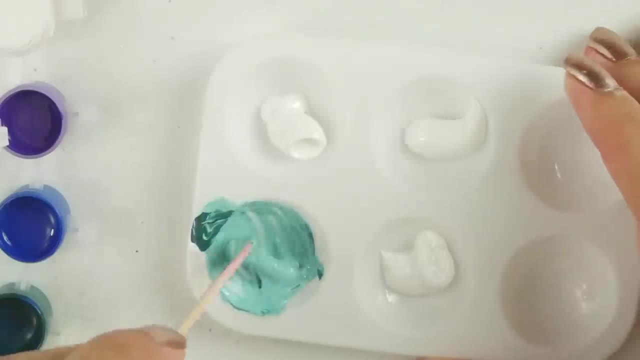 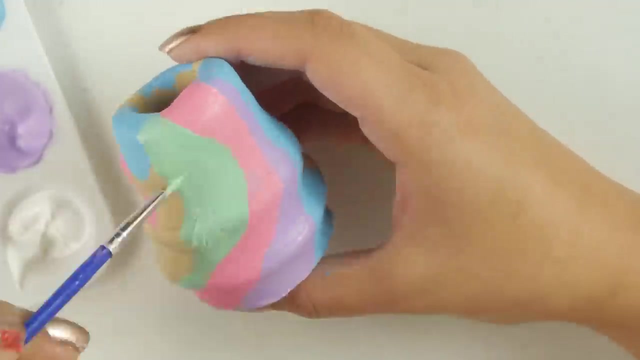 every last bit of the paint they gave me and, as i said, i had to use a lot of my own. i would say it was about half and half, so they give you about half the amount of paint that you need. i will say the quality of the paint actually wasn't that bad. it was nice and opaque. it had a nice shine to it. 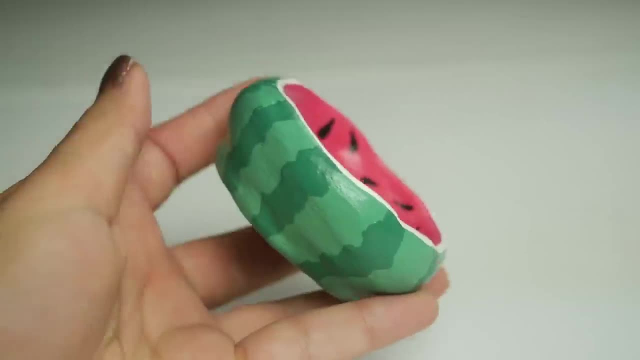 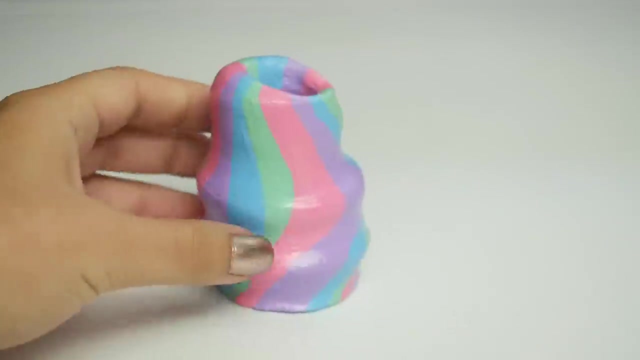 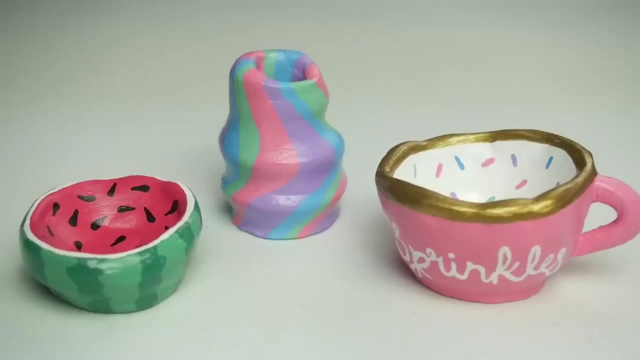 i liked it, honestly, there just wasn't enough of it. so here's what we've got. we got the bowl, which is watermelon themed, the tea cup, which is a sprinkle theme, and this thing. honestly, i have no clue what it is, but it actually may be my favorite. so, yeah, that's, that's them. i don't know. 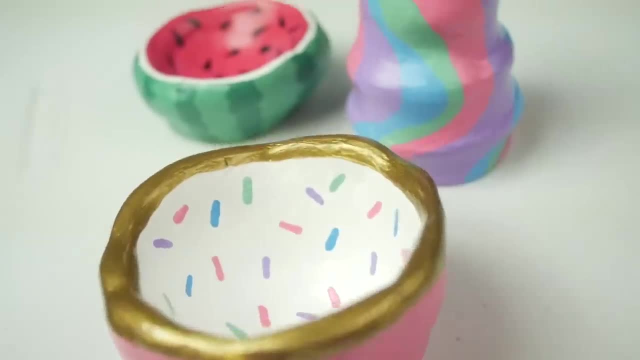 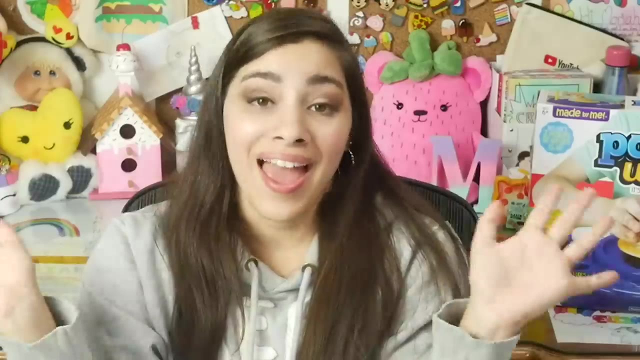 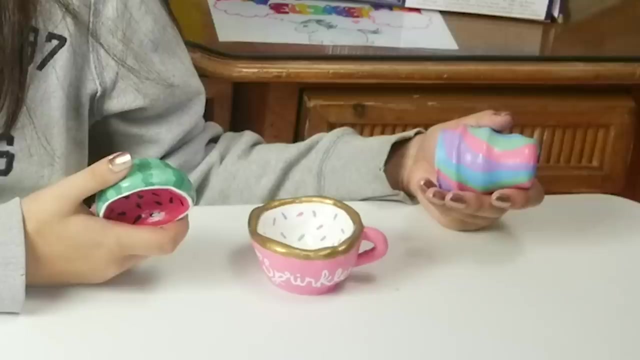 what people are gonna say about these. clearly, i know they're not the best, but maybe you can at least see what i was trying to do or appreciate the effort. hey, this uh video took me- like what, three days to film. this is what i have to show for it and, yes, that means i haven't changed my 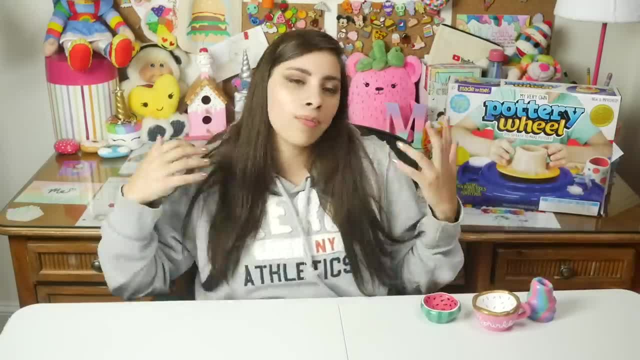 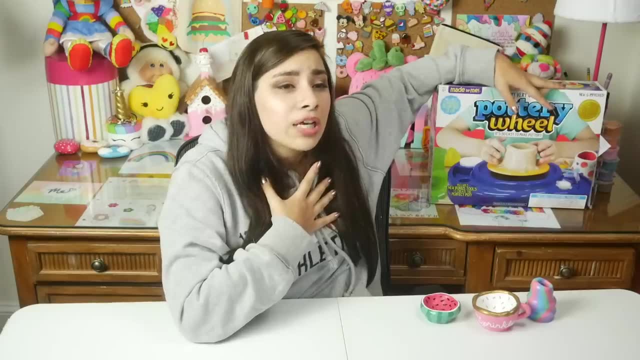 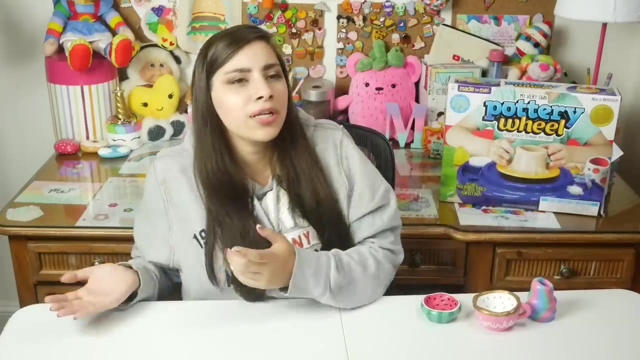 clothes or showered in three days. i'm just kidding, i just put this back on because consistency- my experience using this kit as a beginner- um, even after reading through the instructions thoroughly twice, was a nightmare. but since i have no experience, nothing to compare it to, i wasn't sure if it was just me. 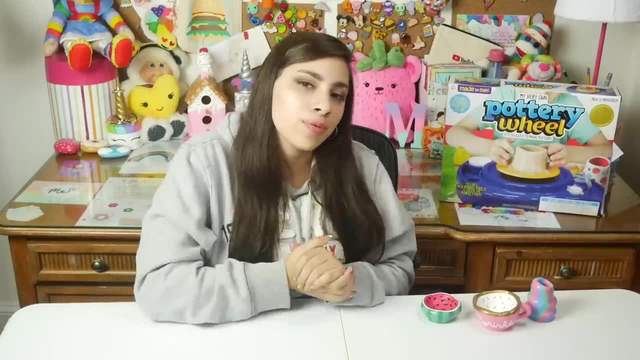 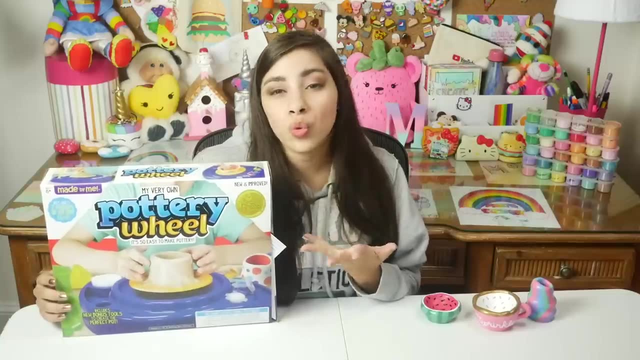 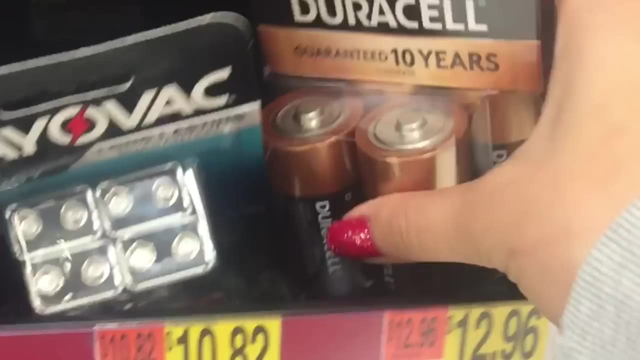 or if the kit just sucks. so after doing some research i realized that this is basically the worst pottery wheel on the market. i mean, it's twenty dollars compared to like a beginner's pottery wheel, which is closer to eighty. but then again you do have to spend like thirteen dollars on batteries, so thirty three dollars actually. 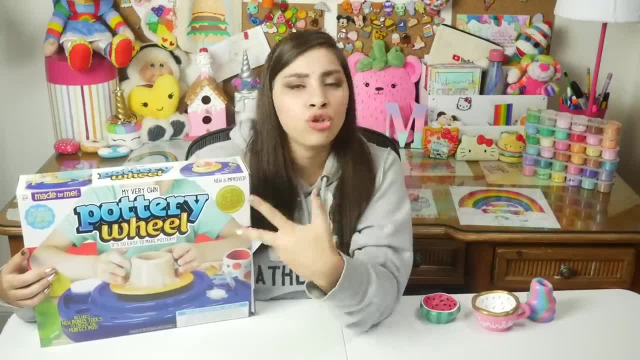 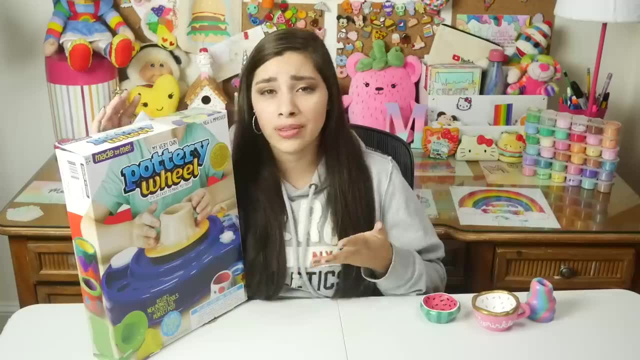 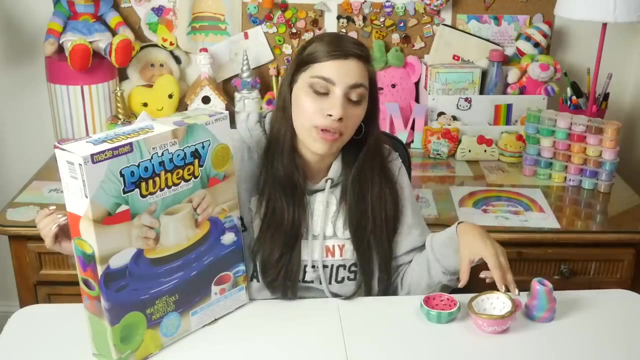 okay, stop making that face. now. it has a stunning two star rating on amazon. that's a terrible rating. so i went on youtube. i looked for other people doing the same kit. most people had similar results to this kind of quality, although they were kind of hyping it up and being like 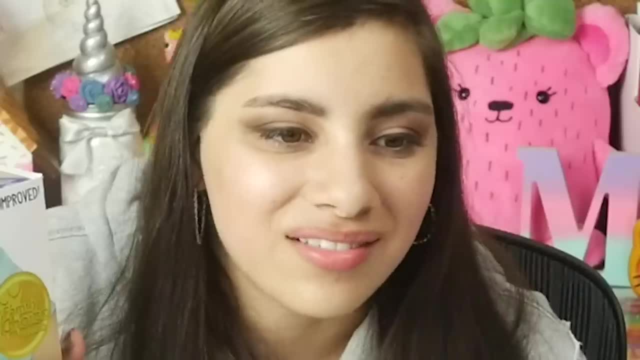 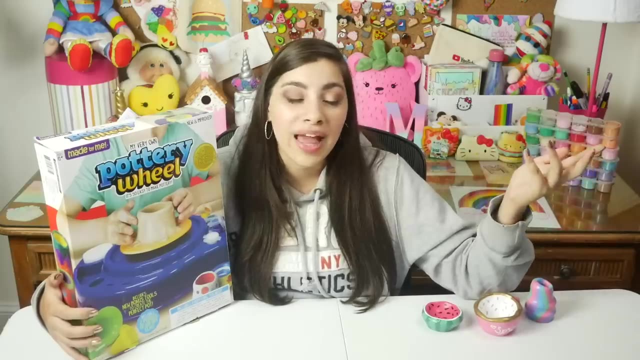 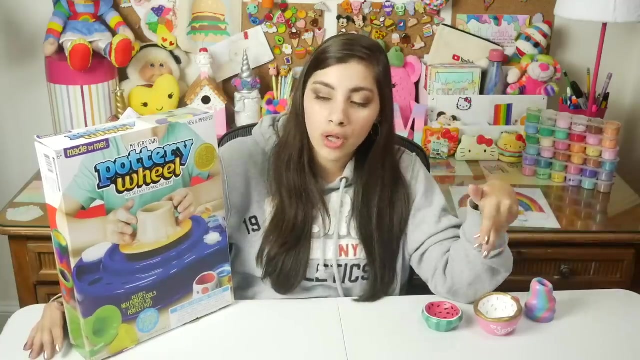 oh, yeah, it looks so great. no, it doesn't. but i did find a legit review from a woman who actually does pottery and she basically knew just by looking at it that it was going to be terrible. okay, that's gonna make a wobbly pot, yeah, and she did have a lot of the similar struggles that i had. i've managed to crack a. 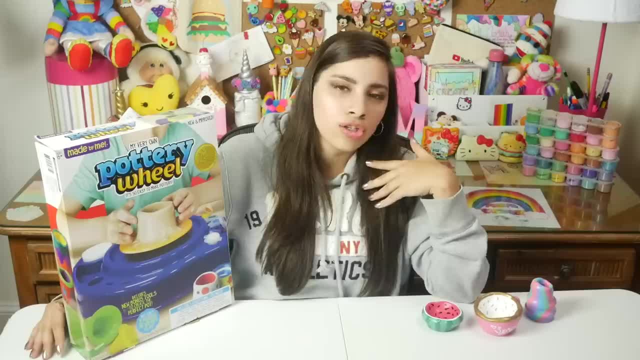 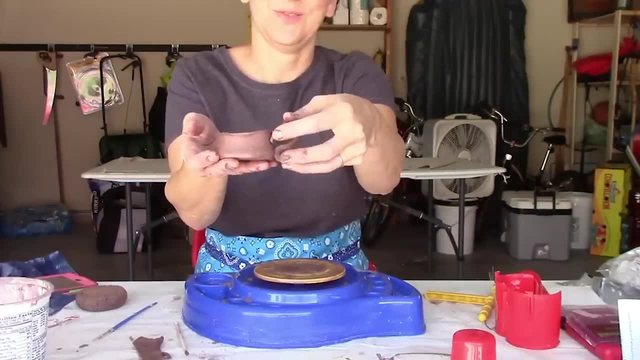 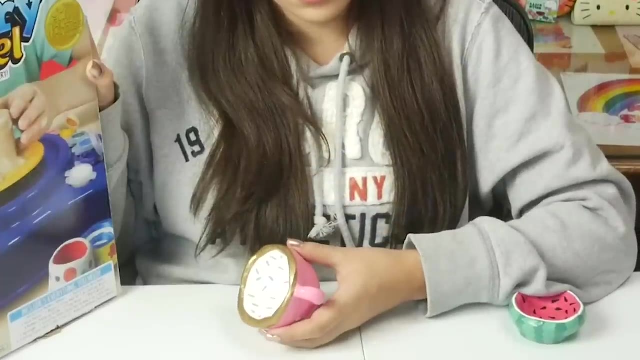 hole right through the clay. yeah, so i felt better until i saw what she made. i think it might be this clay, so i'm gonna switch sweet teacup. if you're a beginner at pottery and have no clue what you're doing, you're going to be very